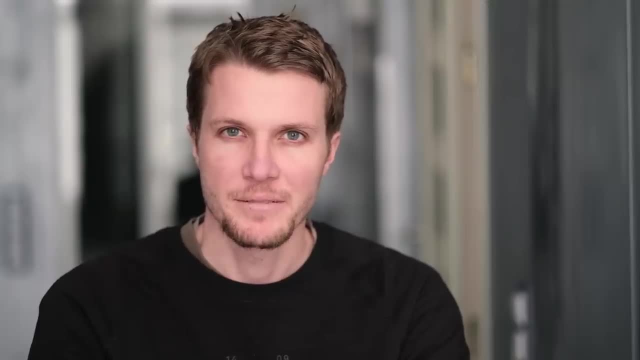 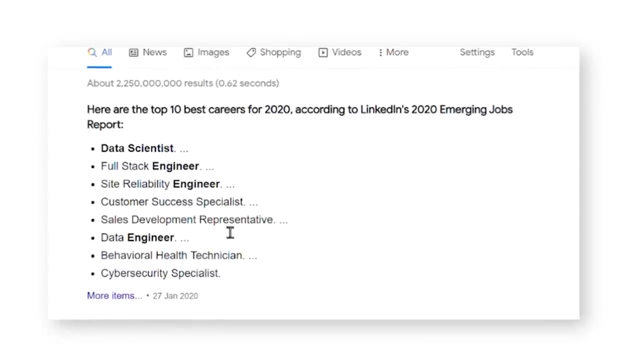 Stage one, the beginning. You're unhappy with your current career. You want more money. You just want to try something new. So you go to the source of all truth and knowledge, googlecom. You type in the search bar: best careers in 2020.. And on every single list, one job seems to come. 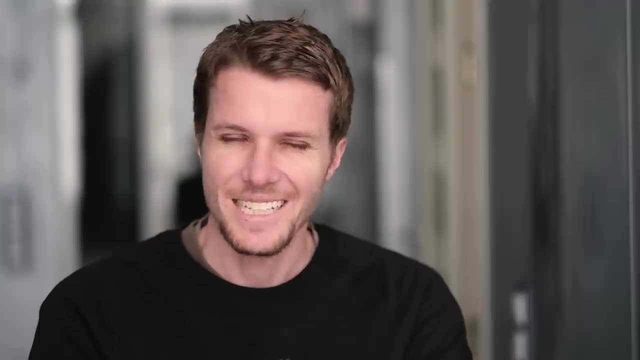 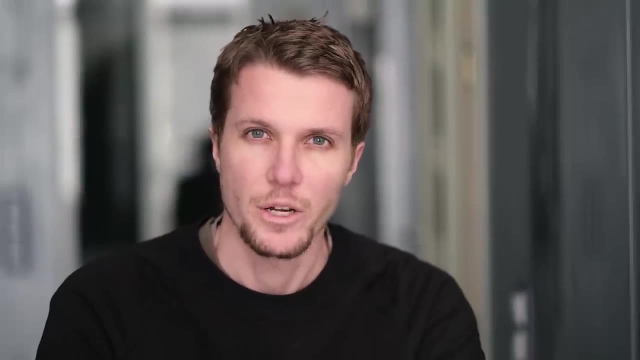 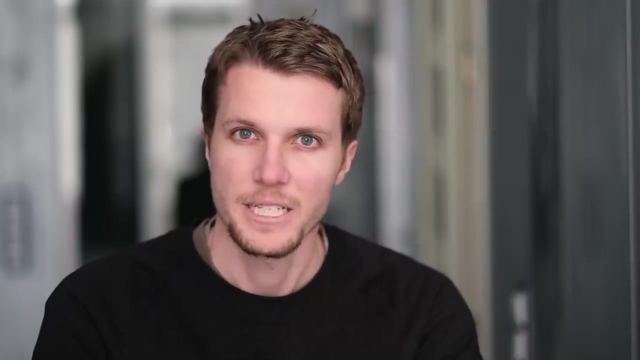 near the top Software developer. That's kind of like HTML, right. But then you have the big moment. Maybe it's on Reddit, a YouTube video or on a coding bootcamp website. You read the single line: You can do this without a college degree and get a job at a top company. 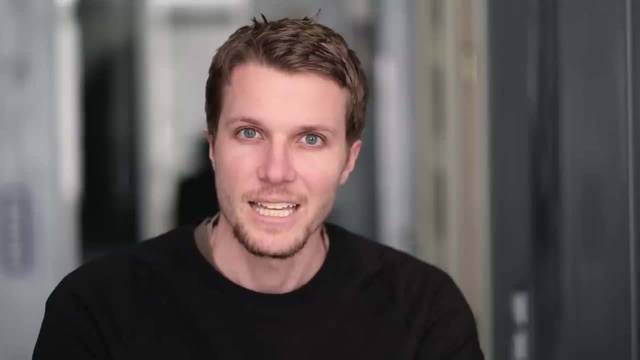 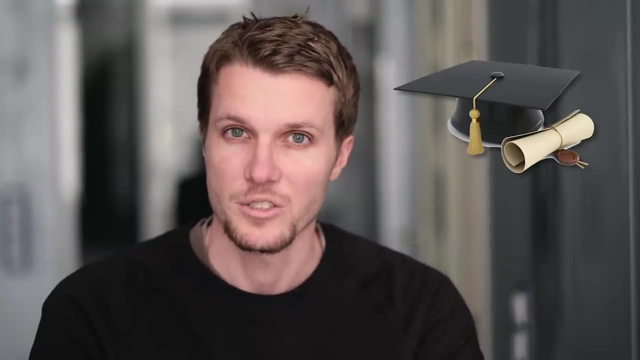 like Google or Facebook or go directly to freelancing and live anywhere you want. It's not just that you don't need a computer science degree. You don't need an engineering degree or a college degree at all. Maybe this is something you yourself could actually do. 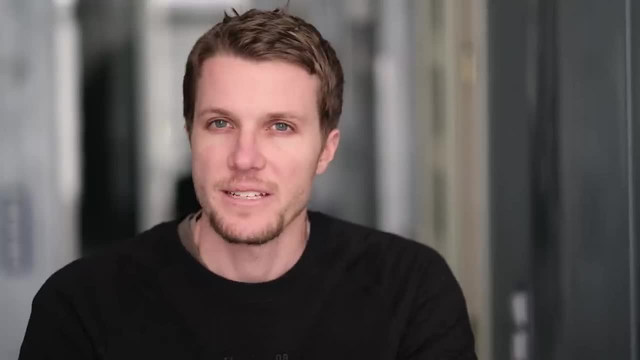 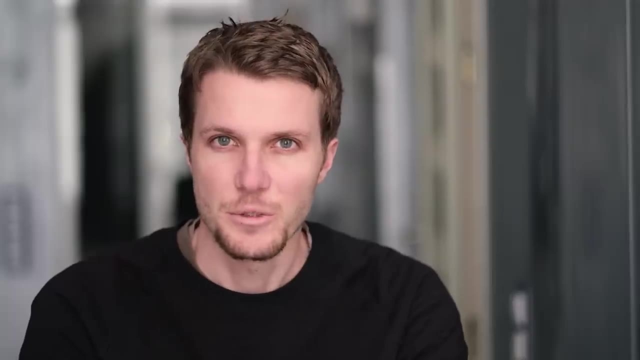 Have an interesting job, make more money, work remotely And the only thing standing in the way is learning to code. How hard could it be right? Stage two: optimism. So you go straight to YouTube and you find this guy's video Fastest way to become a software. 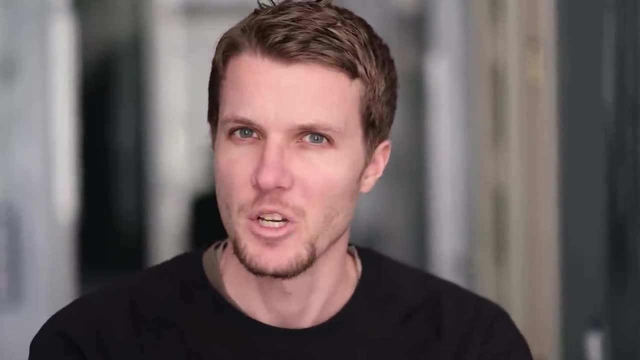 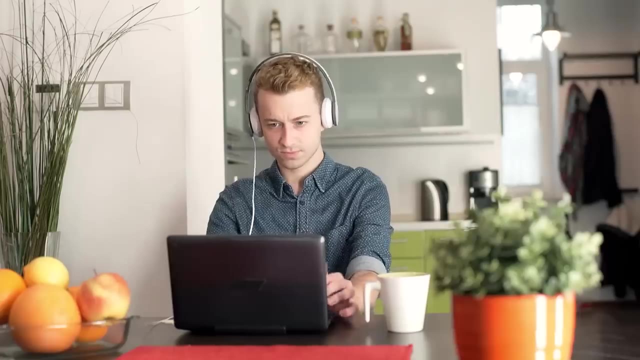 developer. He seems pretty smart and super handsome, So you can probably trust this guy. After that, you start binge watching different channels and they confirm what you suspected before. You don't need a degree and you can actually learn all this stuff online. You start to see that a high salary was just the tip of the iceberg. You can get stock options, free food and you're working on some of the coolest, most unique stuff out there, And you actually get the chance to build software that millions of people would use. 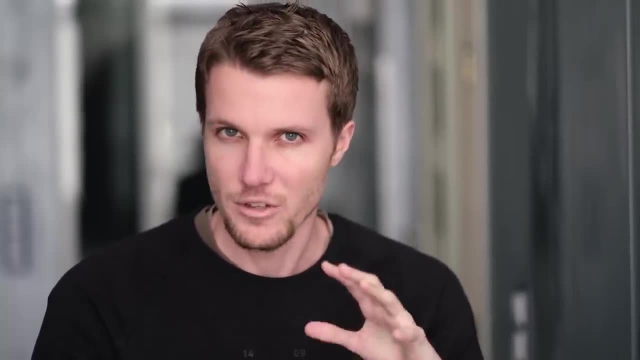 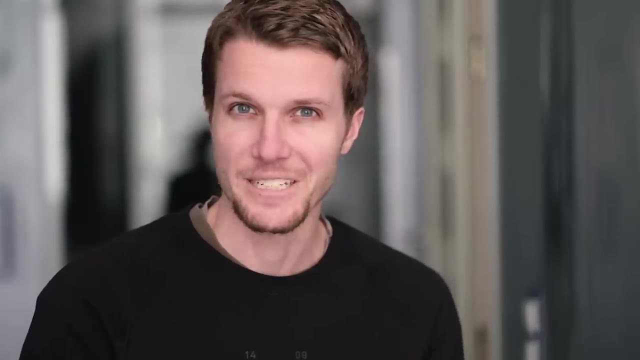 You are now sufficiently motivated, But before all that, you actually have to start learning. So you go and you buy your first tutorial. Damn that actually feels good. How about two, three, four? Let's do all of these and learn this stuff, starting today. 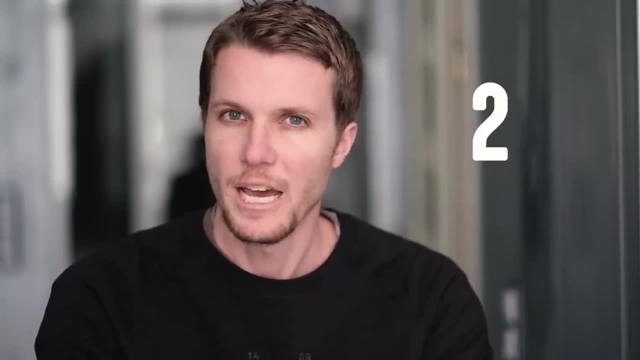 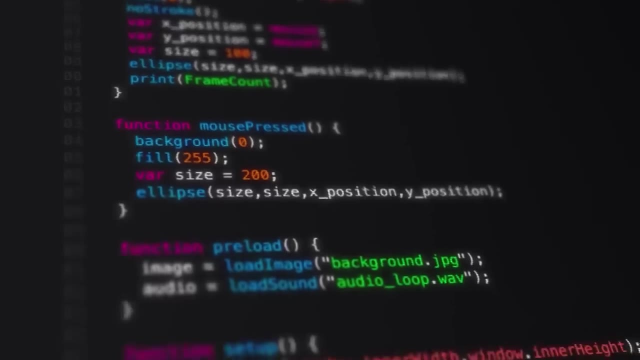 Stage three: doubt. One tutorial down, now two, now three. Feels good to learn Two times speed. why not Feels good to get through it? But then you open up a code editor at the end and nothing, Did that just go? 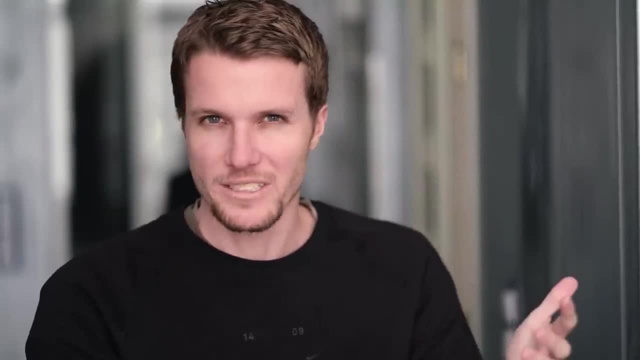 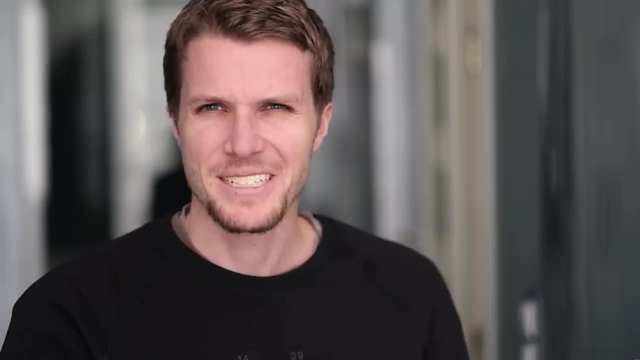 What? Wait, I should know all this. I just watched three courses, But in fact you still can't do anything. So are you dumb? or maybe you should give up, right? Yeah, maybe this is not actually for you. Wait, OK, these courses were probably just bad. 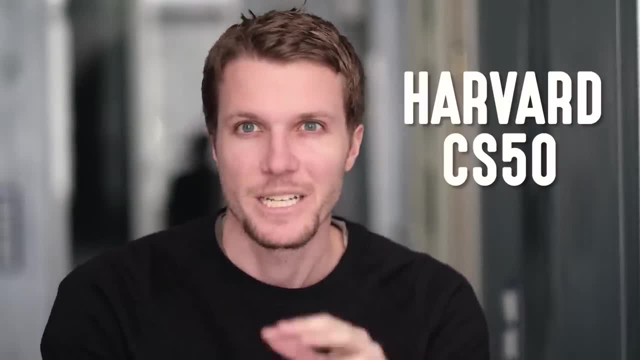 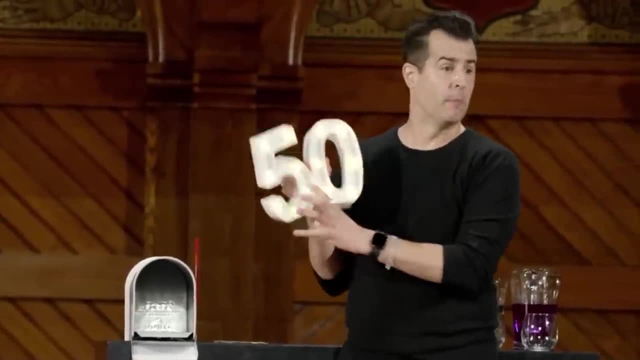 Let's try a real course: Harvard CS50.. This one is super popular, super well-reviewed, So let's do it. And it does seem really high production quality. You should have started with this one, right. OK, time for homework number one. 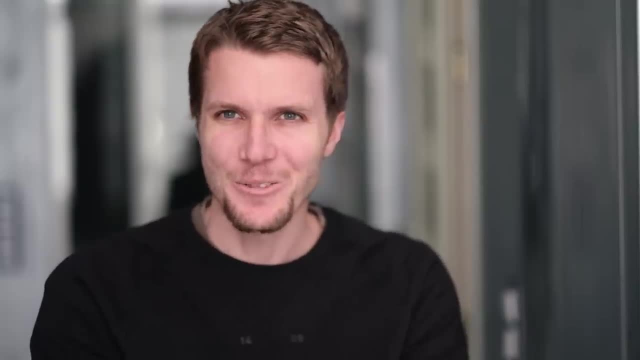 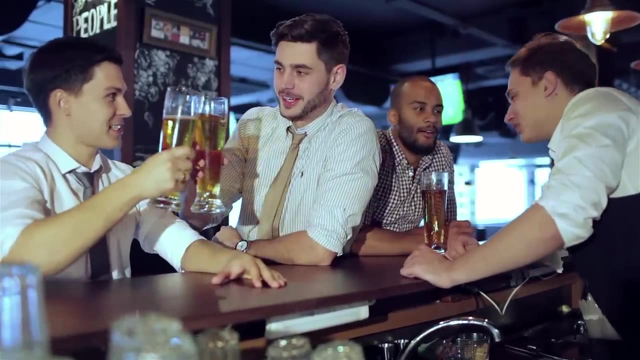 Wait what? This is impossible. How does anyone do this? And this is the first one. This is way too hard. Now you start to rationalize. You'd rather do something more relaxing after your job than learning to code. It's not really worth your time. 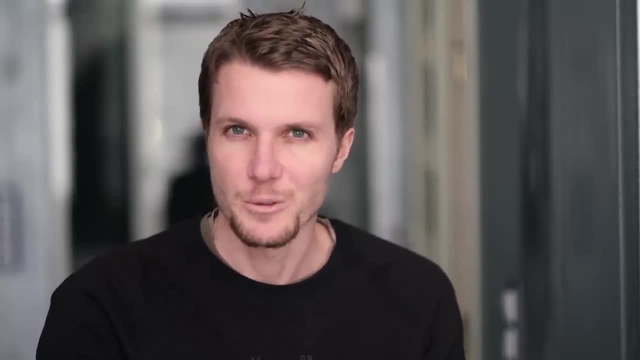 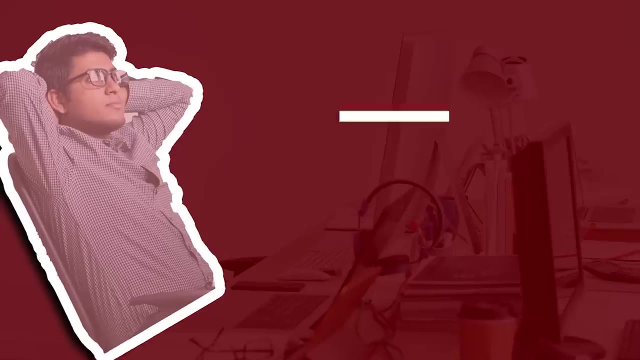 These kind of thoughts get very appealing, Unless you're one of the lucky few who doesn't have a plan B. Maybe you're already rock bottom. In that case, only one way to go forward: Stage four: confidence. And just when you're finally about to give up, it happens. 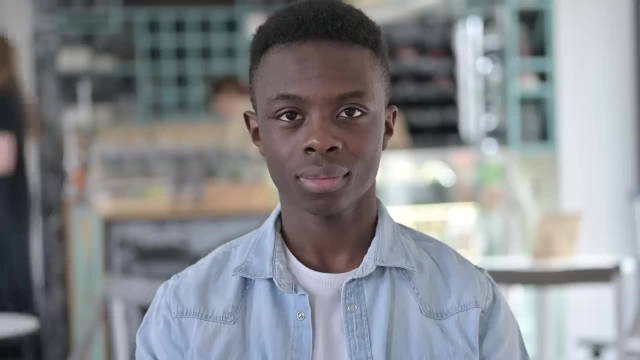 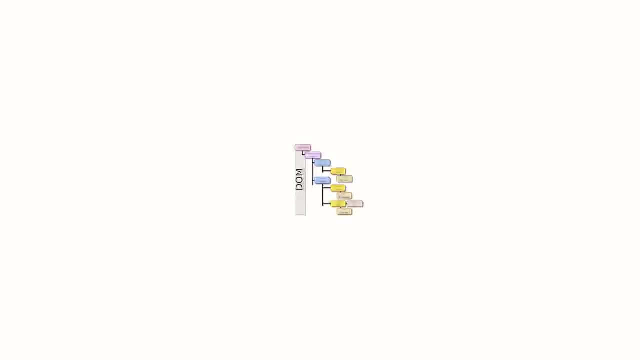 One small thing clicks and you finally get that feeling, that spark of dope meat. Yes, Maybe it's solving your first code wars problem and then solving your second one. All of a sudden, the browser DOM, which seemed really complicated, you realize is only a few commands over and over again. 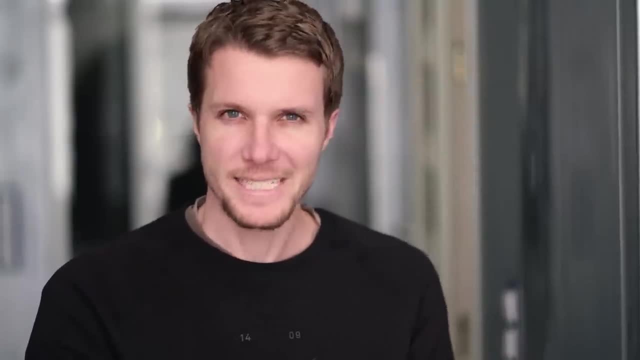 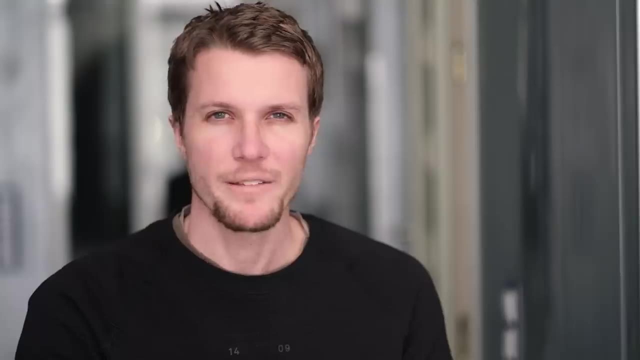 Same with promises: They used to be hard, but they work the same way every time. Oh, that CORS error again. Yeah, you already saw that before. Reverse an array- Don't make me laugh. What previously seemed like an endless list of topics eventually runs. 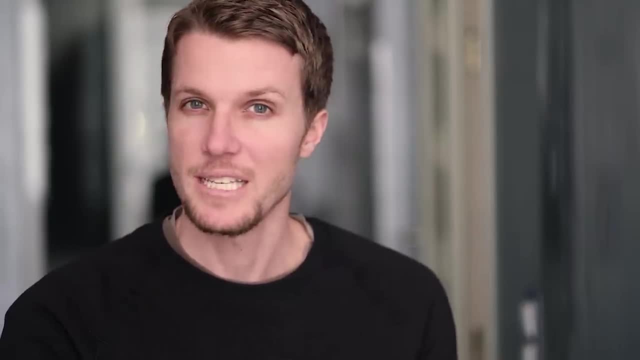 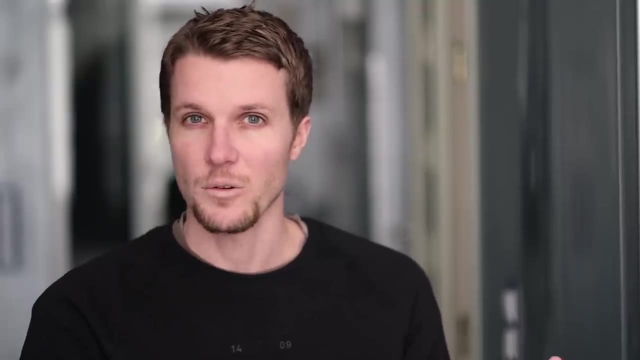 out. Now you've covered pretty much everything, and every project you build gets a bit easier and a bit faster. Stage five success: Now you're building full projects on your own, consulting the docs or a little tutorial here and there where you need to, but you're feeling pretty good. 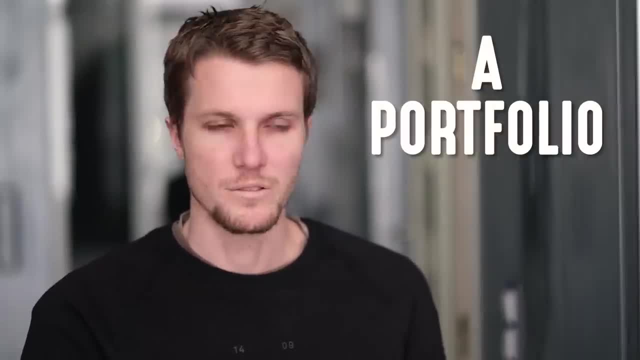 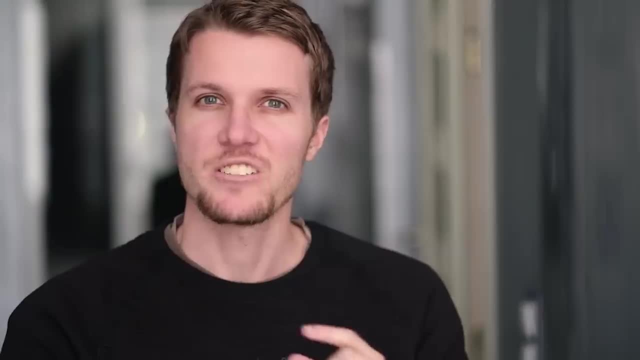 Actually good enough to put together a portfolio. So what's left now? Well, are you really ready to start applying for jobs? So you dust off your resume, throw all your projects on there and change that LinkedIn headline to software developer- Damn, can you really just start applying now? 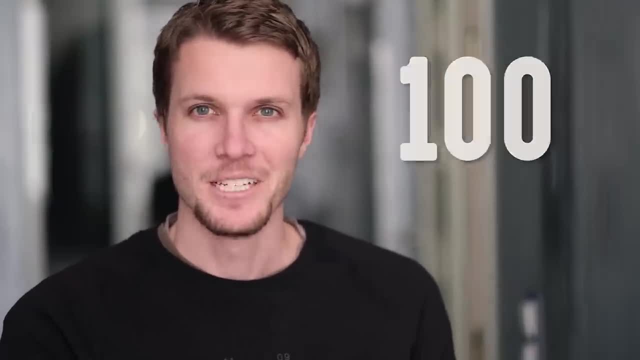 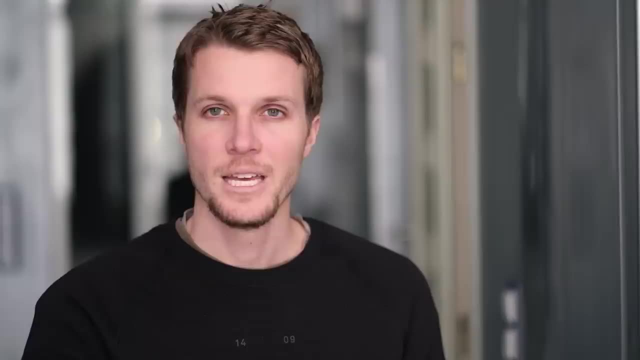 So you do? you send out 10,, 20, 100 apps. Okay, you're not getting much of a response, but you still need to prepare for interviews in the background, learning a bit of data structures and algorithms, And, before you know it, you get that first email back.